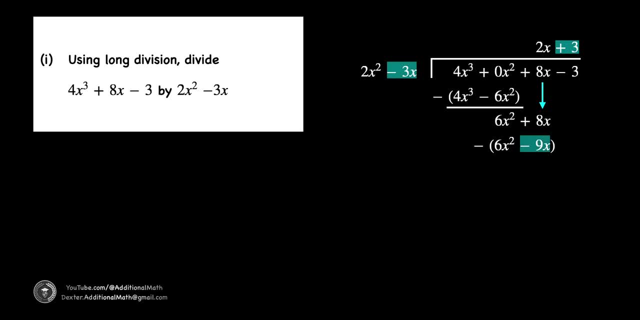 Then we multiply 3 by negative 3x, which will give us negative 9x. Subtracting 6x square minus the 9x from the sum of 6x square and 9x will give us 17x. We will complete the long division by bringing down the constant of negative 3.. 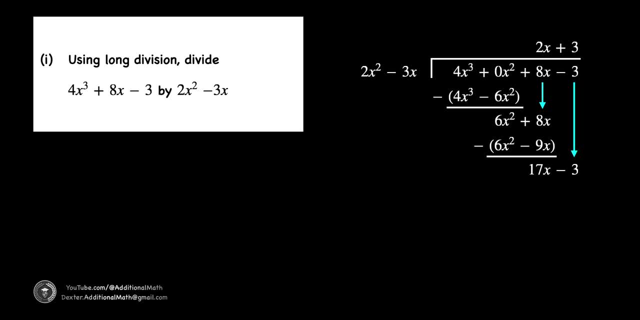 The long division process will end when the remainder can no longer be divisible by the highest exponent in the divisor. The long division can be summarized by having a dividend divided by the divisor, And the result will be the quotient and the remainder, thus dividends divided by divisor. 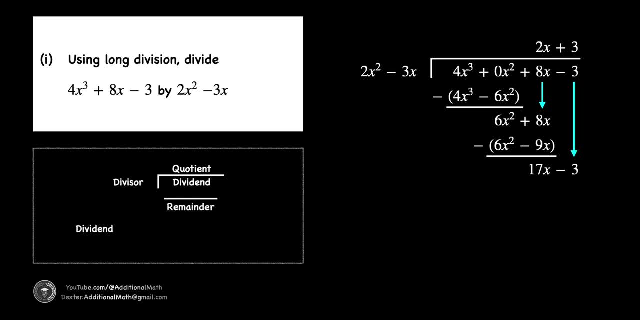 And the result will be the quotient and the remainder, Thus dividends divided by divisor. the long division will be reduce to x and dx. etaping the long division process- consumers to live longer with 0x and y in the longer term- is called interviews. 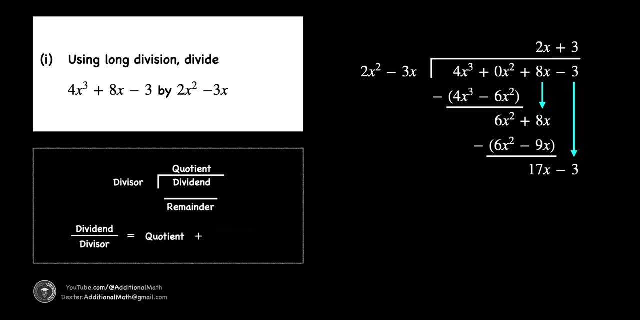 divisor will be equal to quotient plus remainder divided by divisor. The division algorithm can also be obtained from this by multiplying divisor throughout this equation. Our answer can therefore be expressed as 2x plus 3, which is the quotient plus 17x minus. 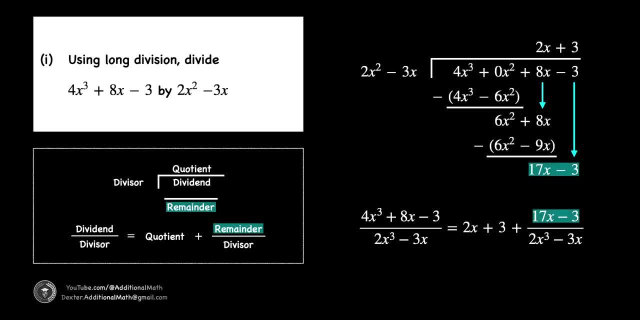 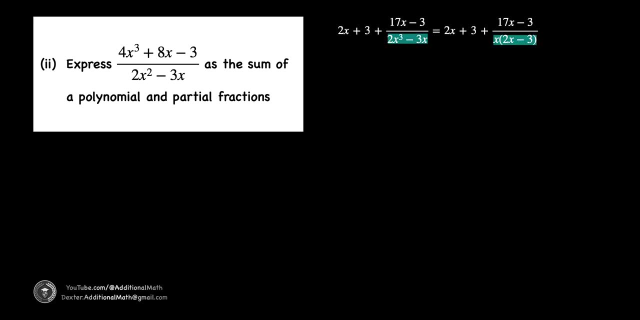 3, which is the remainder divided by 2x cubed minus away 3x, which is the divisor of the long division, And that will be the answer to part 1 of this question. We will begin part 2 by factorizing the denominator of 2x cubed minus away 3x into the product. 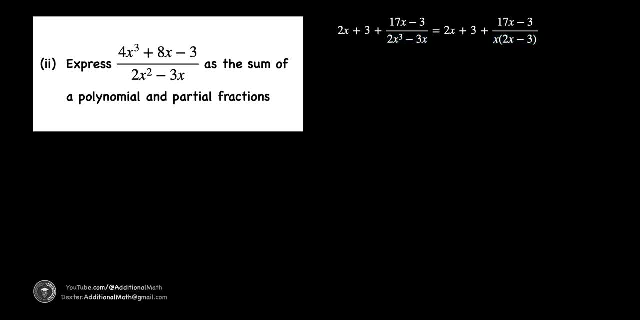 of x and 2x minus 3.. For the decomposition into partial fractions: if the denominator contains distinct linear factors, such as the product of ax plus b and cx plus d, we can express the partial fractions as a divided by the first linear factor plus 3x. 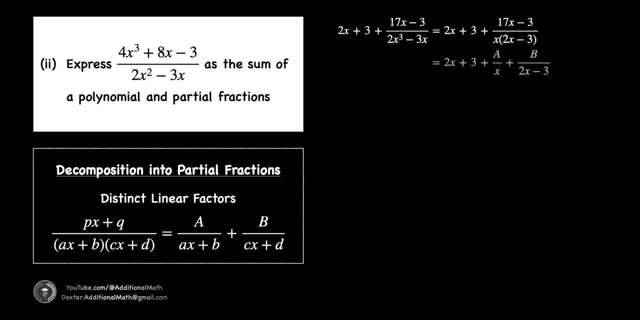 We can also write the partial fraction as a plus b divided by the second linear factor. It means that for our first distinct linear factor, x in the denominator, we can write it as a over x, And for our second linear factor, 2x minus 3, we can write it as b over 2x minus 3.. 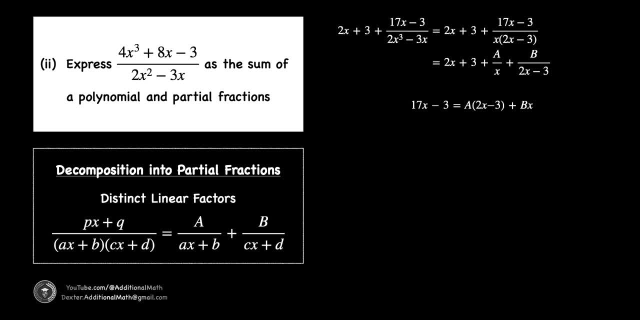 By multiplying the partial fractions such that we have a common denominator of x and 2x minus 3, we will form this new equation: To get the same common denominator, we will take the product of constant which is negative 3a, Then we multiply b by x.